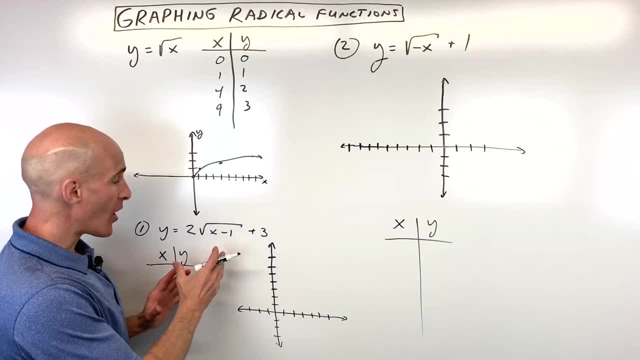 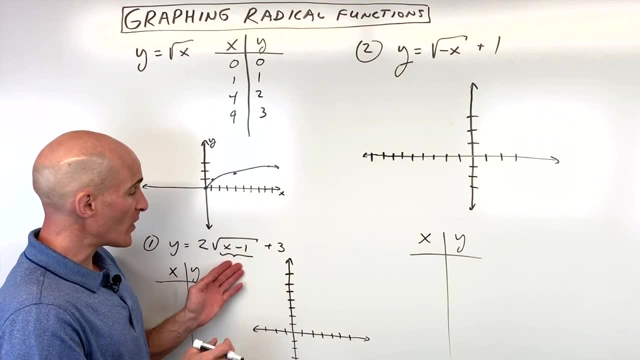 That's our basic graph. Now, the method I'm going to show you here is how to use these key points to get the graph of a more challenging square root function. So, taking a look at what's underneath the square root, we ask ourselves: how can I make this equal to 0,, 1,, 4,. 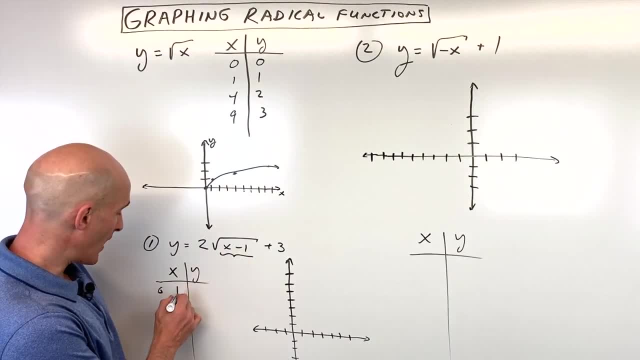 and 9?? Well, in order to make this 0,, this would have to be 1.. In order to make it 1,, this would have to be 2.. In order to make this 4,, this would have to be 5.. In order to make this 9,. 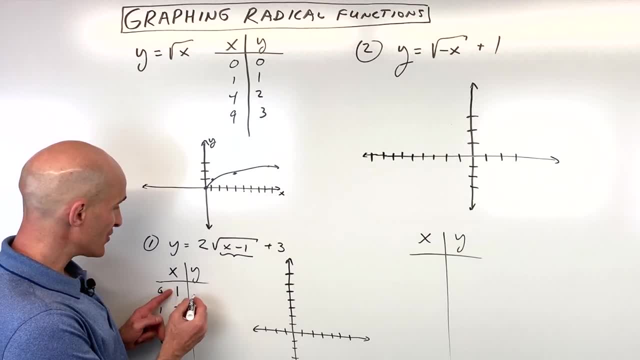 this would have to be 10.. And so now we're going to use these values and you can see we're going to get: square root of 0 is 0, times 2 is 0, plus 3 is 3.. If we put 2 in, we get 1.. Square root of: 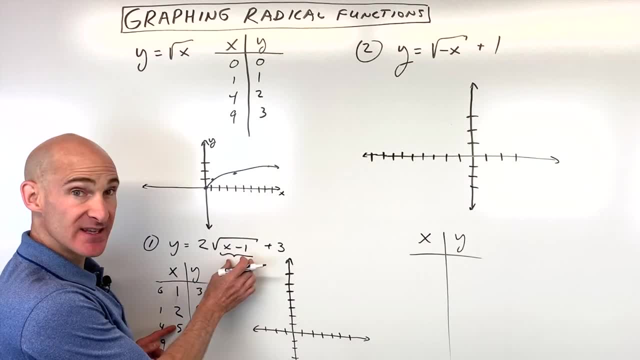 1 is 1, times 2 is 2, plus 3 is 5.. So we're working from the inside out. 5 minus 1 is 4, square root of 4 is 2, times 2 is 4, plus 3 is 7.. And then 10 minus 1 is 9,. 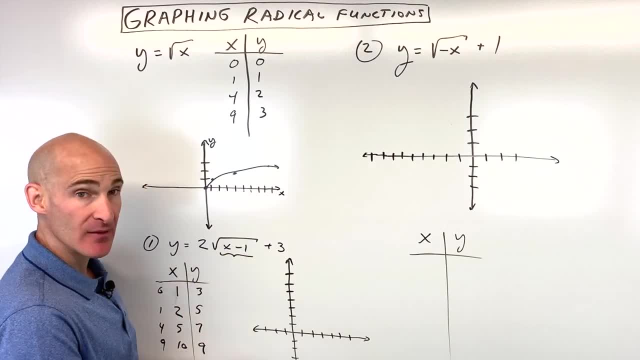 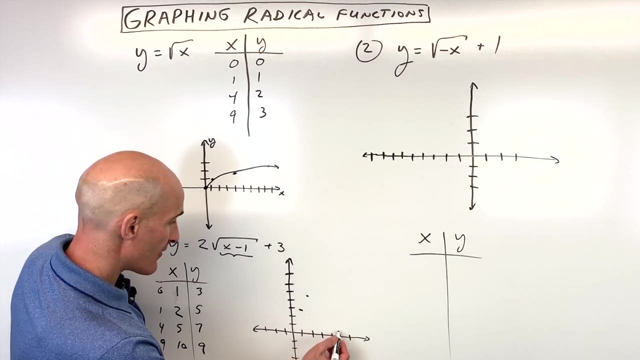 square root of 9 is 3 times 2 is 6 plus 3 is 9. so now we can plot those points and get the graph of our square root function and that's going to look something like 1, 3, 2, 5, 5, 7. so 2, 3, 4, 5, 7, let's. 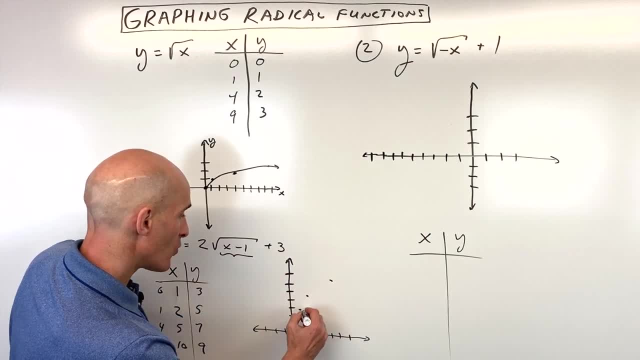 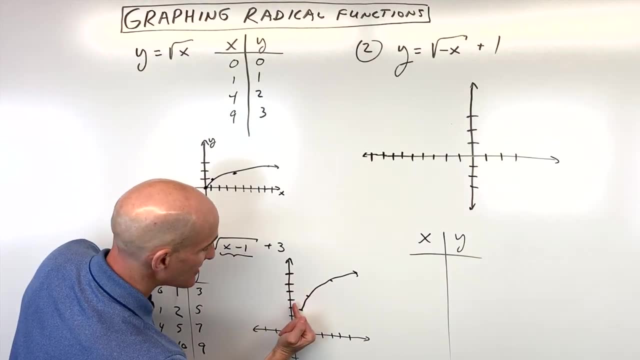 see 1, 2, 3, 4, 5, 6, 7- right about here- and so on, and notice that the graph only goes the one direction. it's not like a line where it goes both directions. so your domain here is going to be: x is greater. 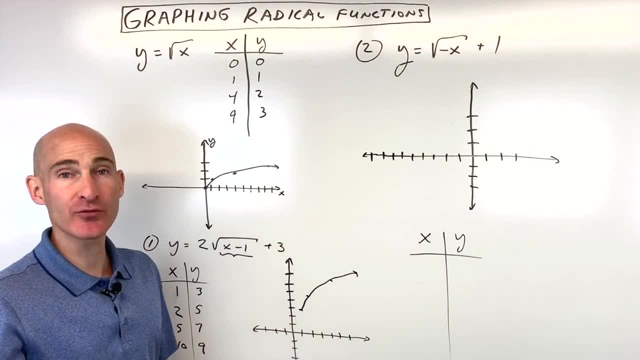 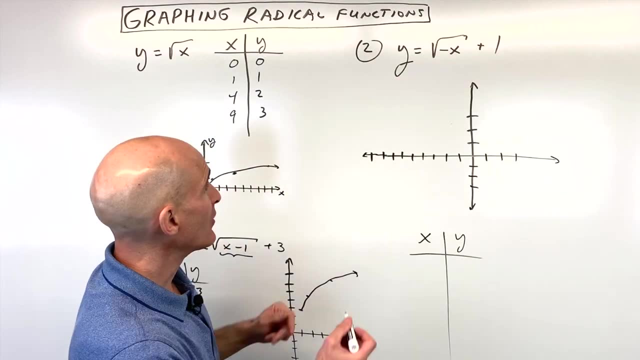 than or equal to 1, and your range is going to be: y is greater than or equal to 3. so let's take a look at another example. say, like number 2, here y equals square root of negative x plus 1. now again, we can use that same technique of making a table. we want to get these values that are easy to take. 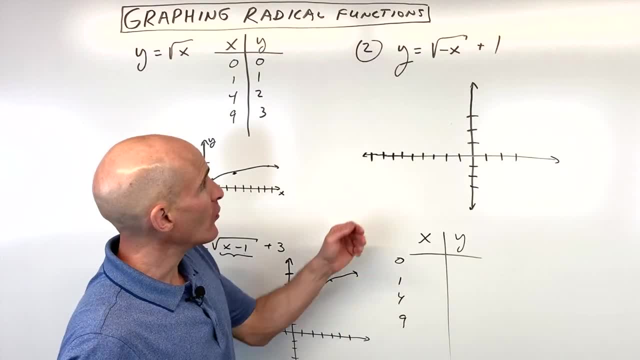 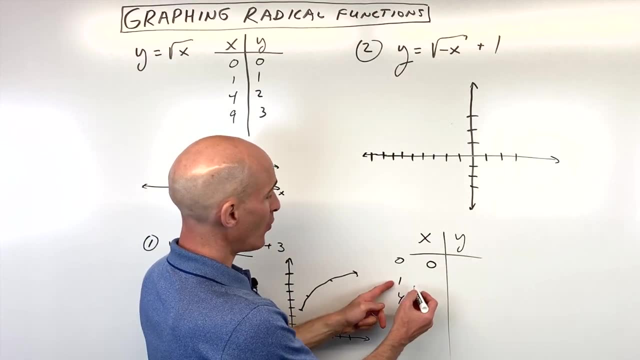 the square root of like 0, 1, 4 or 9. so when we say to ourselves, okay, well, what's the uh? what would make this equal to 0? that would, of course, be 0. what would make this equal to 1? that would be. 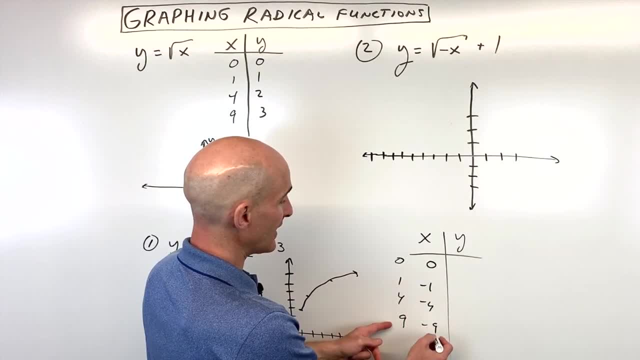 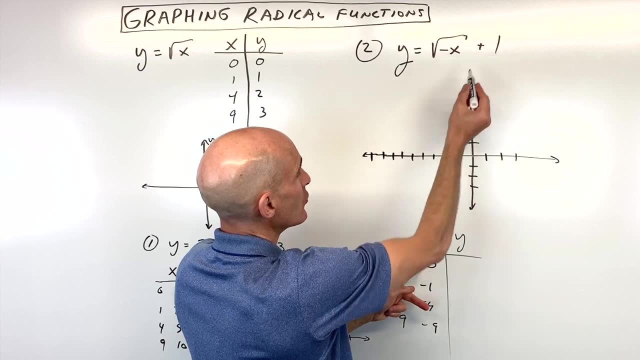 negative 1. what would make this equal to 4? that would be negative 4 and negative 9. so these are going to be our inputs, or our x values. now, when we put them in, we get 0. square root of 0 is 0 plus 1 is 1. negative times: negative 1 gives you positive 1. square root of positive 1 is: 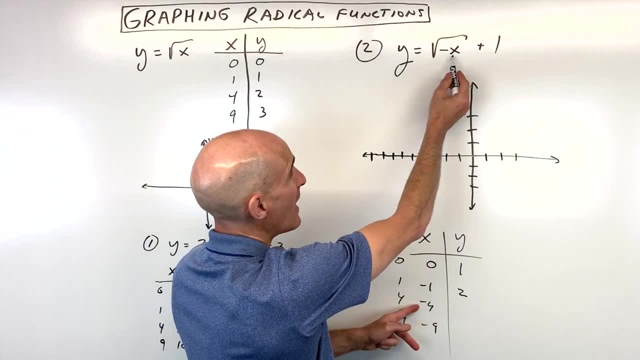 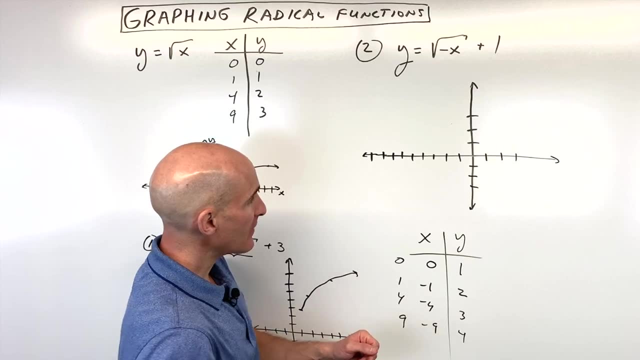 1 plus 1 is 2. negative times, negative 4 is positive 4, square root of positive 4 is 2 plus 1 is 3 and square root of 9 is 3 plus 1 is 4. so if we plot these we can see we're getting 0, 1 negative, 1, 2. 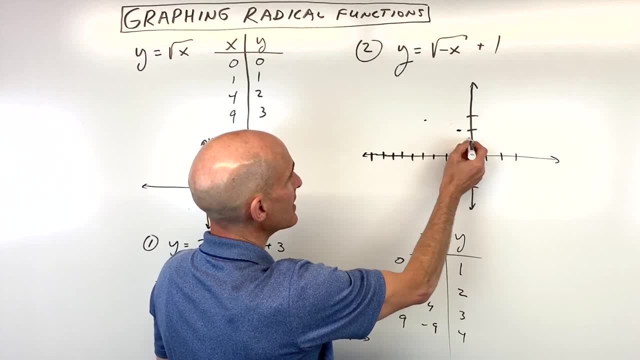 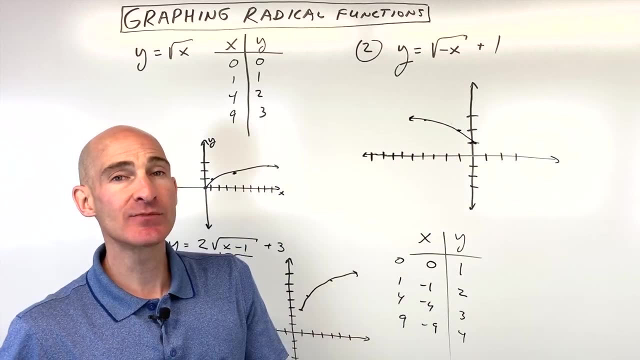 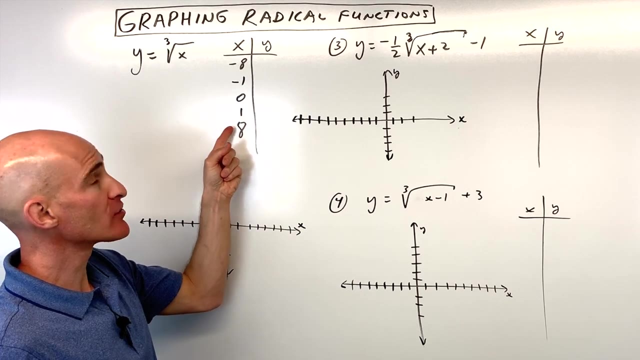 negative 4, 3, etc. and you can see there's. this graph is actually going to the left. this negative is actually reflecting it over the y-axis. now let's take a look at some cube root function. okay, the numbers that you want to really remember for cube root functions are negative: 8. negative 1, 0, 1 and 8, and the reason we remember these ones. 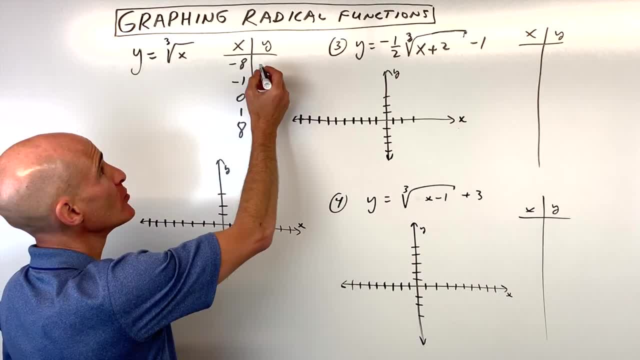 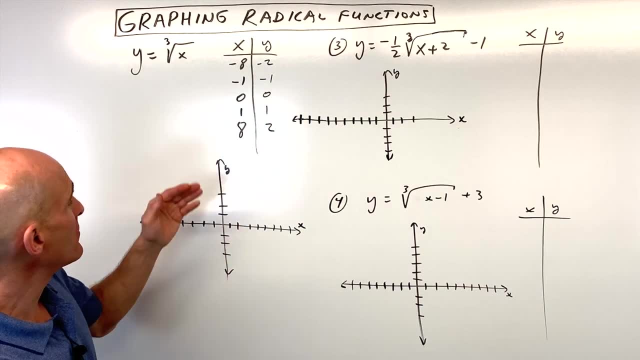 is because it's easy to take the cube root of these values. so cube root of negative 8 is negative 2. cube root of negative 1 is negative 1, 0, 1 and 2.. so now all we have to do is go ahead and plot these. 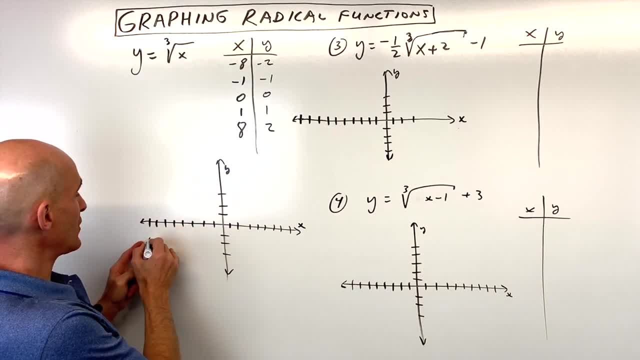 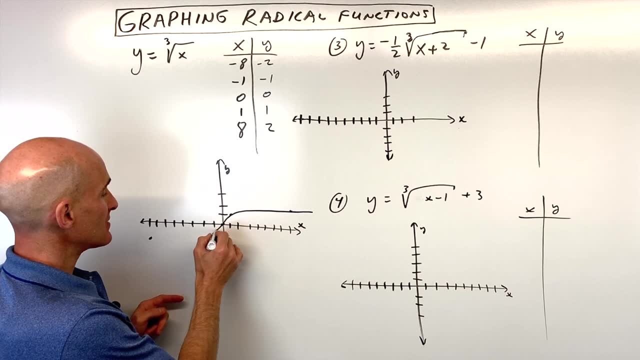 and you can see we're going to get three, four, five, six, seven, eight negative two right about here, negative one negative one here, zero, zero one one and eight two. and you can see we're getting this kind of like s shape graph and the domain is all real numbers. it gradually goes. 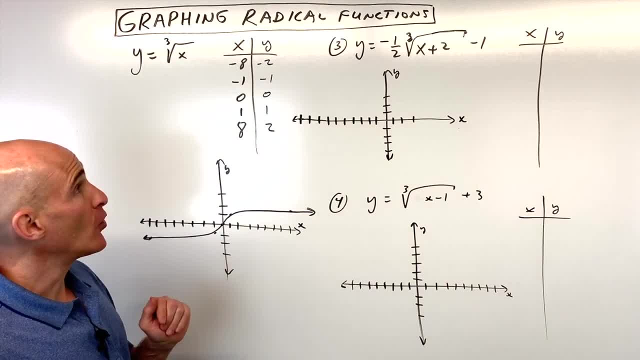 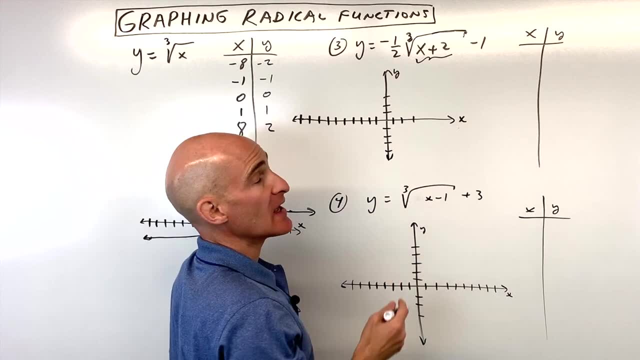 up and down. the range is going to be all real numbers and you've got it. so now, if you wanted to do a little bit more challenging one, like number three again, what you can do is you can look at what's underneath the cube root and ask yourself: what values can i put in for x? 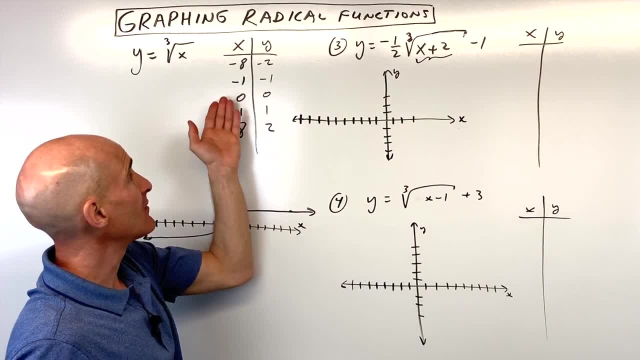 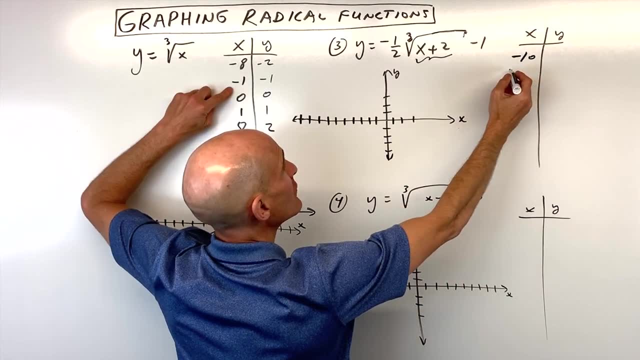 then make this cube root negative eight, negative one, zero one and eight. so it's easy to take the cube root of. so here you can see that we're going to have to make this negative 10 to get negative one. we're going to make this negative three to make this zero. we're. 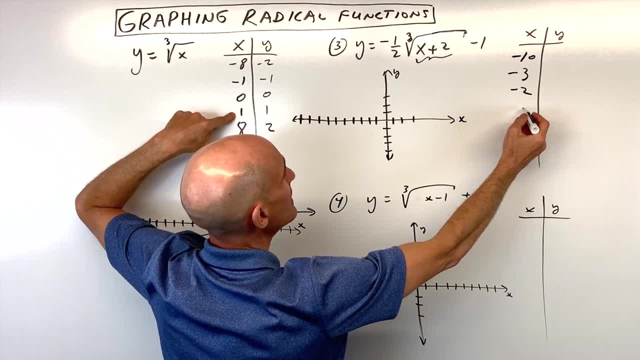 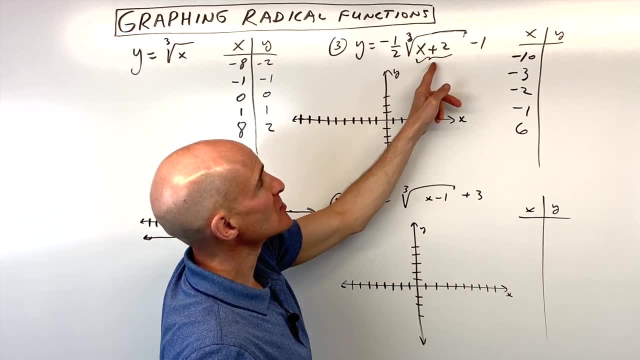 going to get negative two. to make this one, we're going to have to make this negative one, and to make this eight, we're going to have to make this six. so now, when we put these values in negative, 10 plus 2 is negative 8. the cube root of negative 8 is negative 2 times negative. one half is positive. 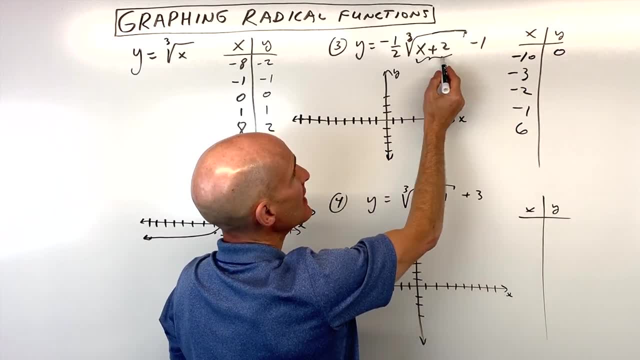 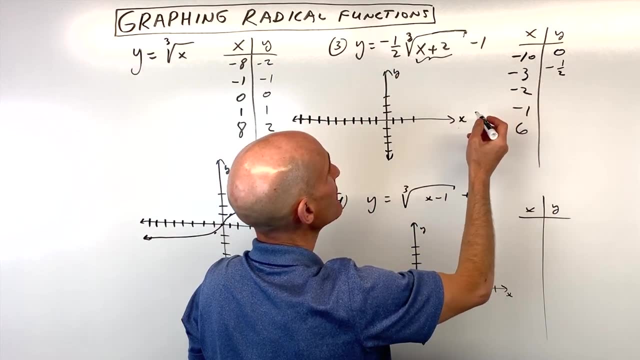 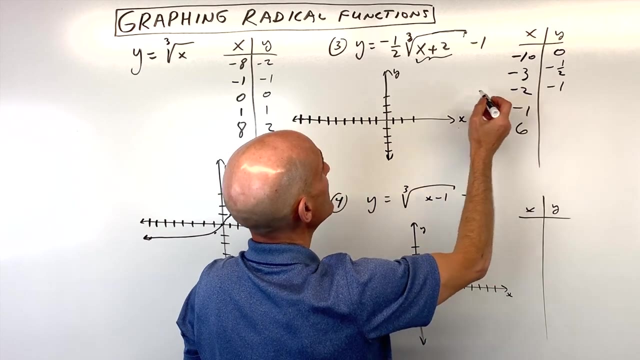 one minus one is zero. if you put negative three, we get negative one. cube root of negative one is negative one times negative. a half is positive. a half minus one is negative a half. if we put in negative two, we get zero, zero. cube root of zero: zero times. this is still zero. minus one is negative one. if we put negative one in, we get 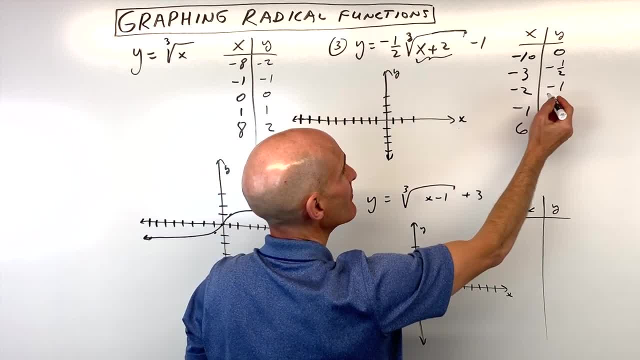 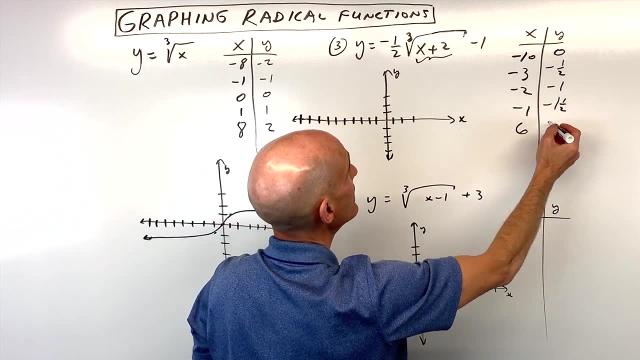 one cube root of one is one times negative. a half is negative. a half minus one is negative one and a half, and if we put in six we get eight. cube root of eight is two times negative. one half is negative. 1 minus 1 is negative 2. so now we can plot these values: negative 10, 0 would be right. 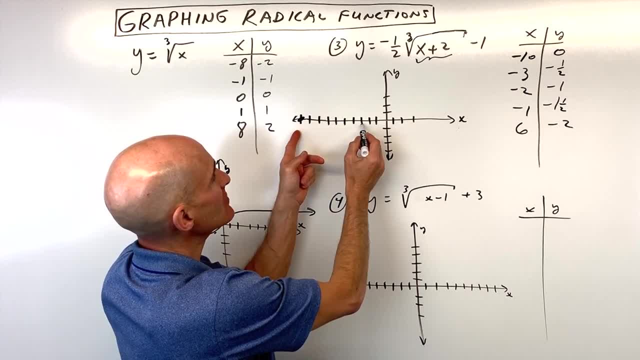 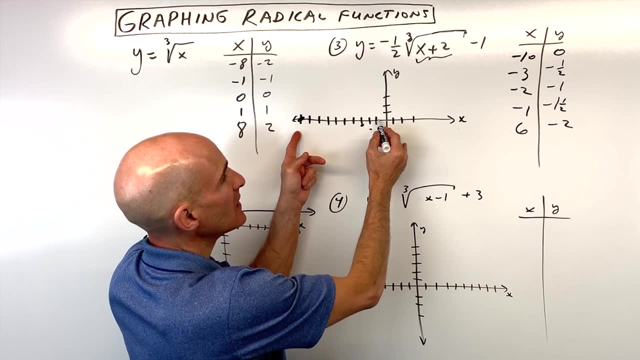 about here: negative 3- negative a half is going to be right about here. let's see, negative 2- negative 1 is going to be right here and negative 1- negative 1 and a half is right about here. and then 6: 1, 2. 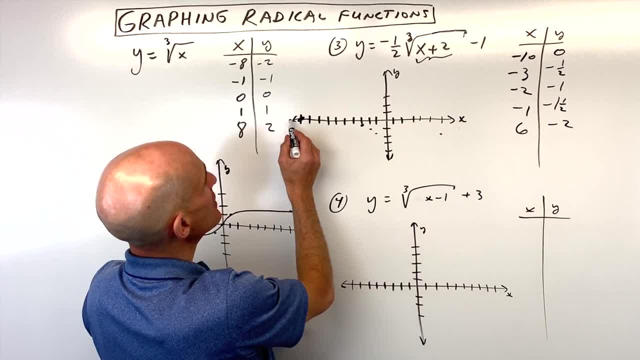 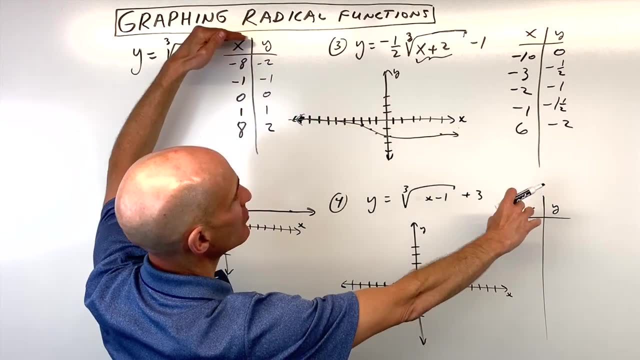 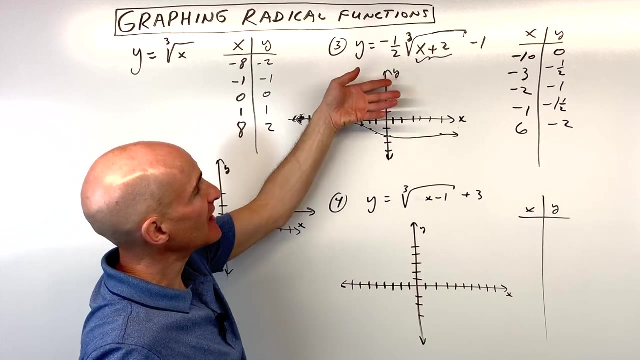 3, 4, 5, 6 and negative 2 is right about here. so you can see this graph is actually looking something like that and it should be going down to the right and up to the right like that. so the domain and range are going to be all real numbers. the one half is compressing the graph, the negative is: 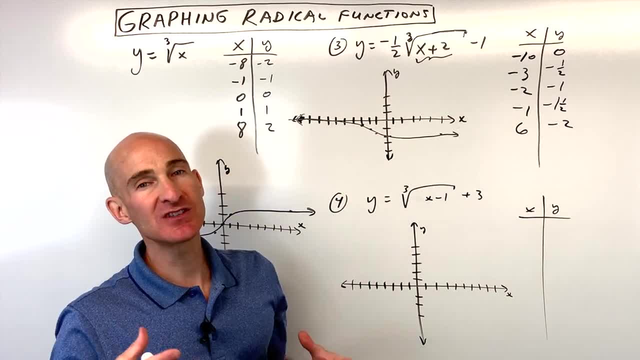 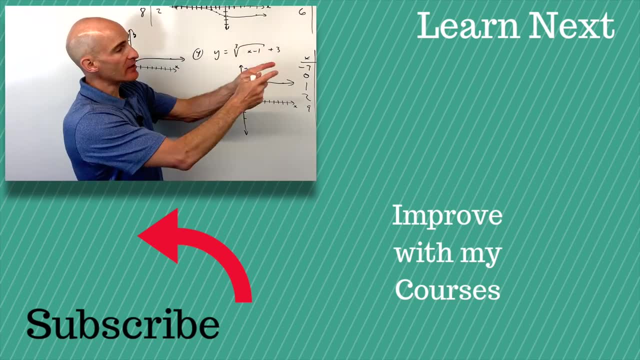 reflecting the graph and these are involved with shifting the graph. but this is just an easy approach. i'm showing you by getting these key values and getting a quick graph. follow me over to that video right there where i'll show you how to graph these using transformations and i'll see.